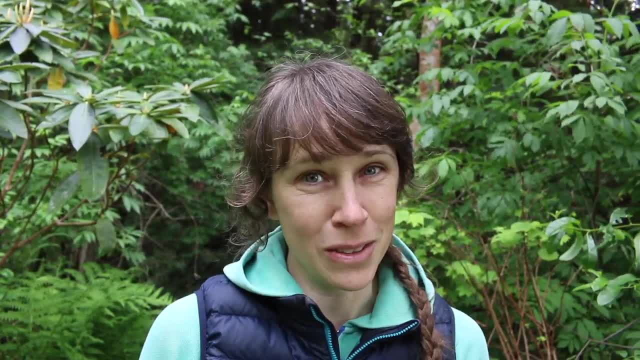 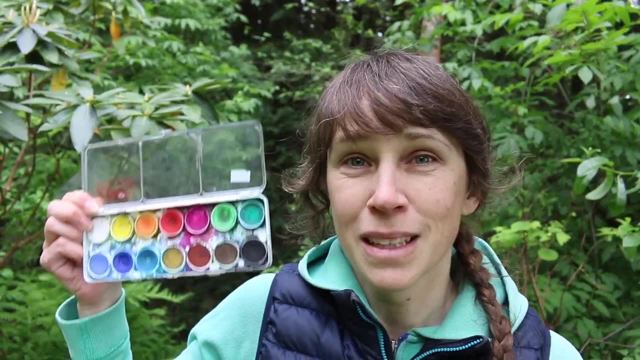 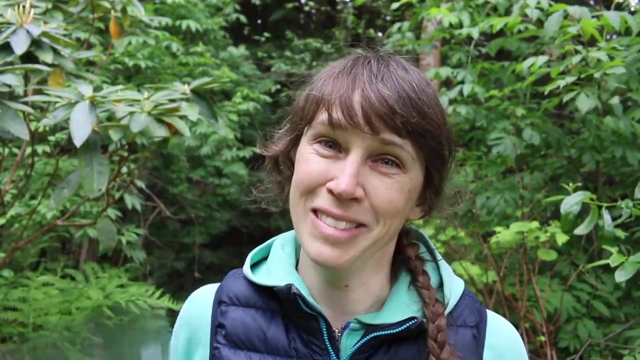 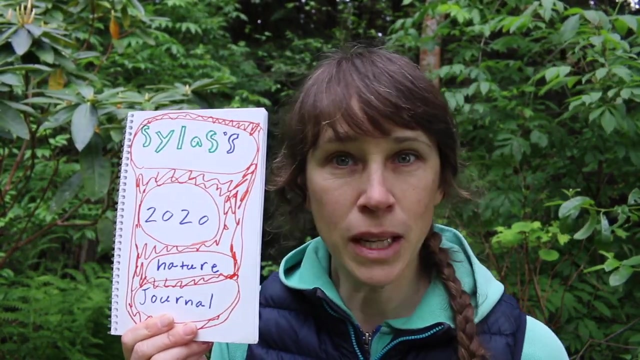 really to collect a palette of colors, Kind of like an artist palette. only the colors we're collecting are not paint, They're colors from things that we find outside. You interested? Okay, let's go. You're gonna need one thing: Your nature journal. You got one Great Bring. 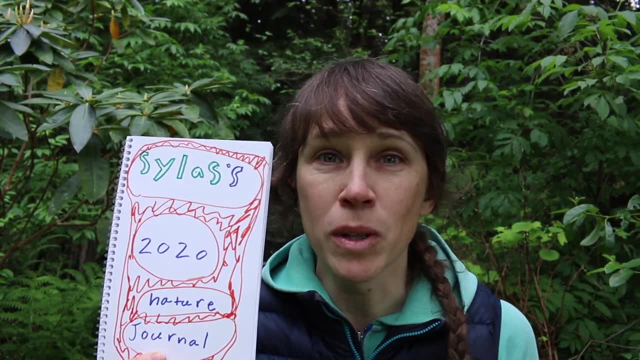 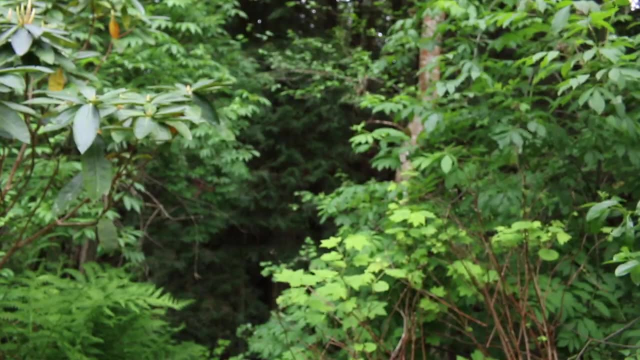 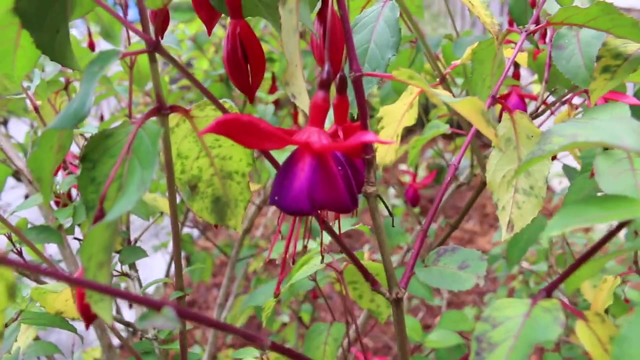 it out. If not, that is totally fine. Grab some paper, maybe a clipboard, Pen or pencil. that helps too. You ready? Okay, let's go. When you start searching for different colors outside, flowers will probably be the first things that you notice, But there are so. 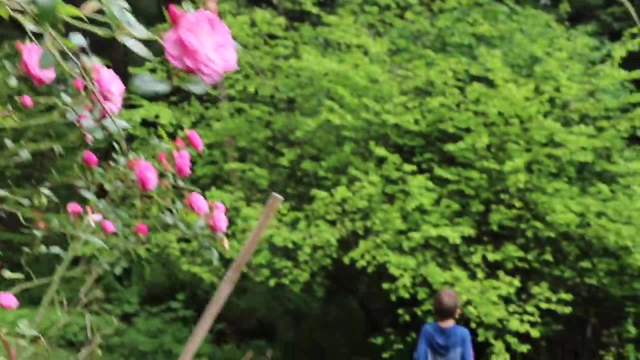 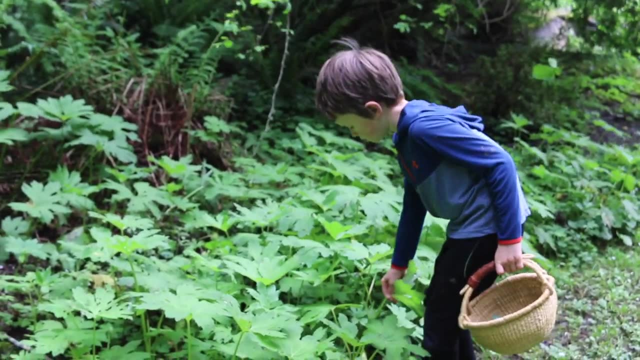 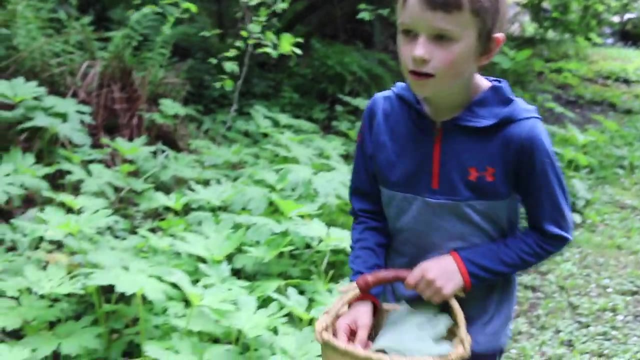 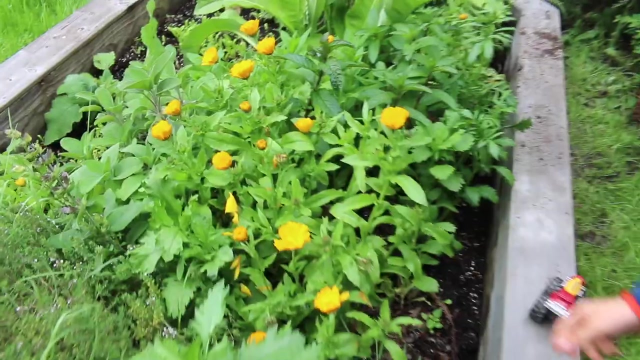 many different shades of green to find too. So I noticed you're getting a lot of green leaves. Do you think that the different green leaves will have different colors when you smoosh them on the paper? Yeah, Guess, we'll see. For this color smash, the challenge is to see if you can collect a whole. 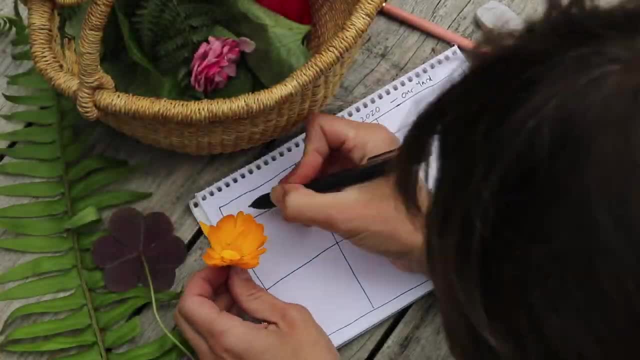 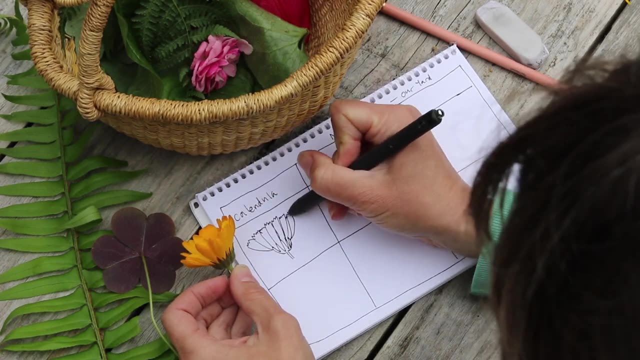 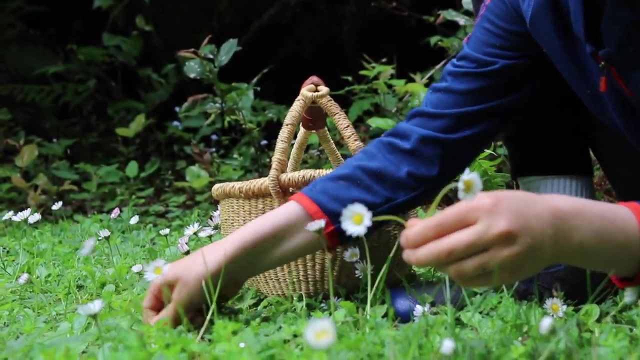 palette of colors from the plants you find outside and keep a record of those colors in your nature journal. How do you do that? By smashing them in there, of course, But more on that in a sec. Your first step is to collect samples, to experiment with. A couple things to be aware of, though. 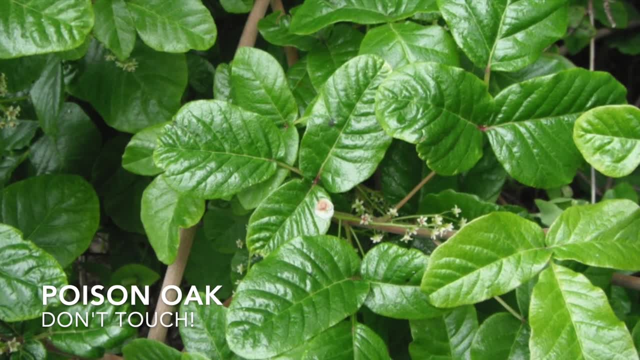 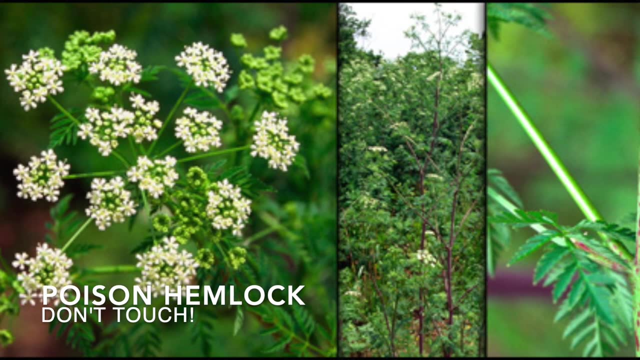 is to make sure you are not touching plants. Some plants can harm you if you touch them, By giving you a rash, a sting, or being poisonous if you eat them. So please be aware of what not to touch in your neck of the woods And definitely wash your hands when you're done with this activity. Okay, 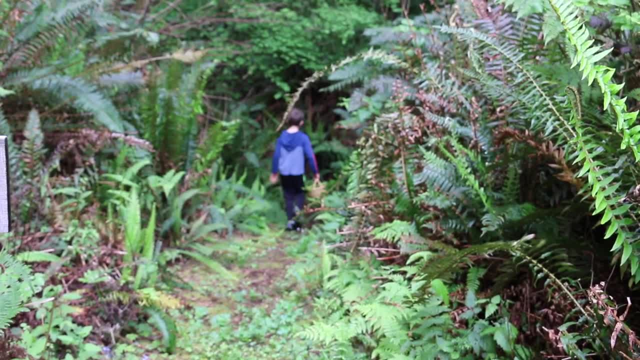 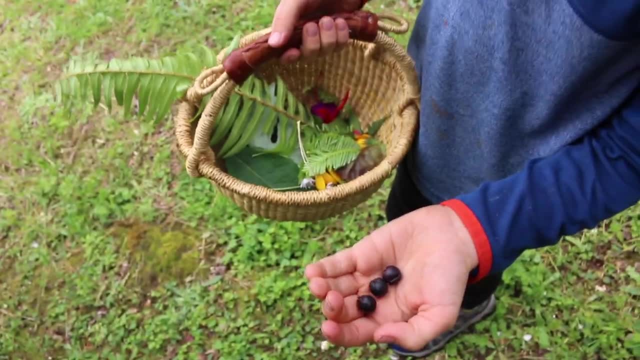 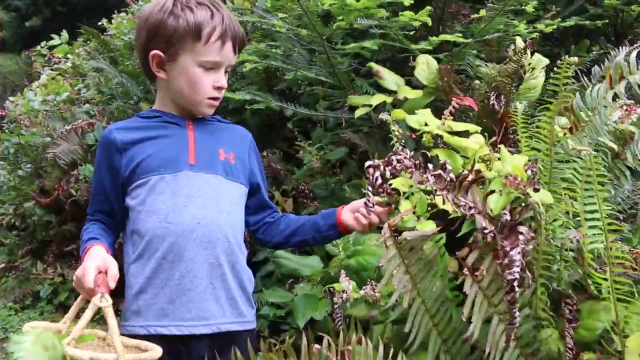 Okay, back to the fun part Time to head outside and collect a variety. That means leaves, flowers, berries are all great. If you're picking flowers, look for ones that are bountiful, have already fallen off the plant. You can try samples of wild plants and those. 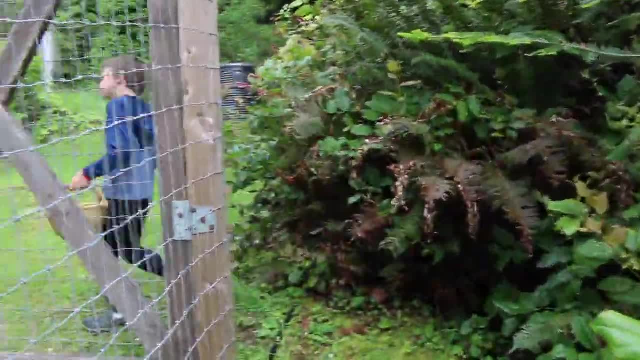 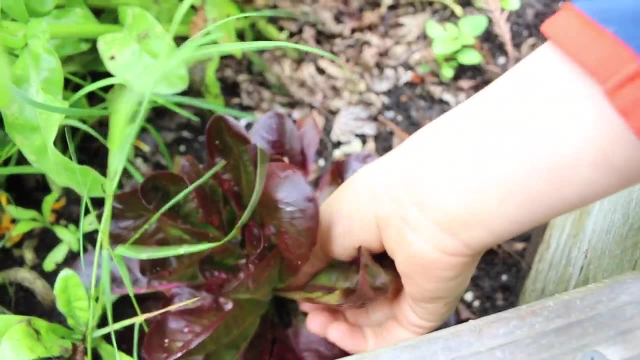 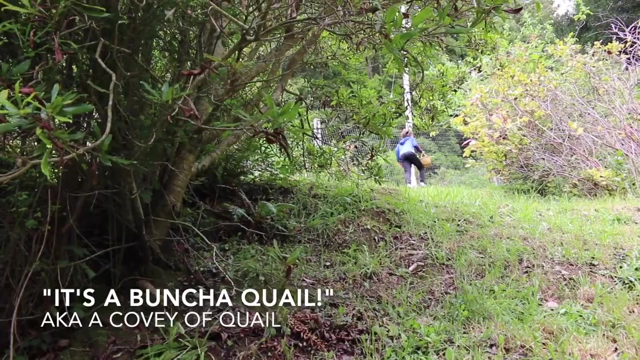 in your garden too. Searching for interesting samples to experiment with is a big part of this activity. What other discoveries do you make along the way while you're at it, And what kind of questions do you have about what you're finding? Here's one.